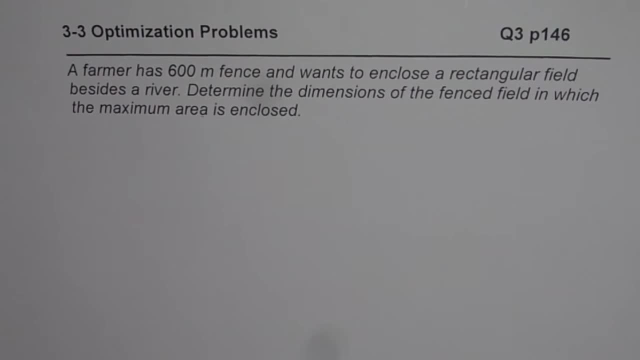 I'm Anil Kumar and on request of my students there is solution of question number 3, page 146. Nelson calculus optimization problems. A farmer has 600 meter fence and wants to enclose a rectangular field besides a river. Determine the dimensions of the fenced field in which? 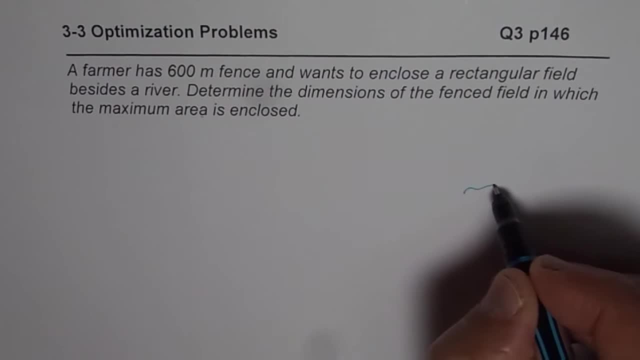 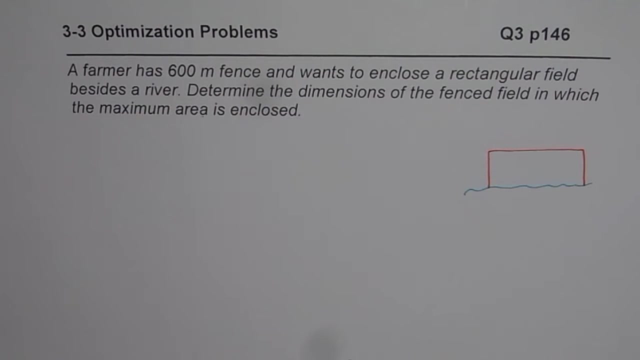 the maximum area is enclosed. So think like this: This is the river for you and the farmer wants to enclose rectangular area. So that is kind of like this. So what you need to understand here is that the fence is applied only in three sides, Right. So let's say: 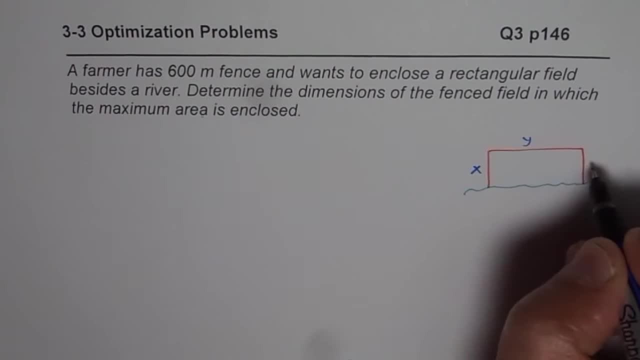 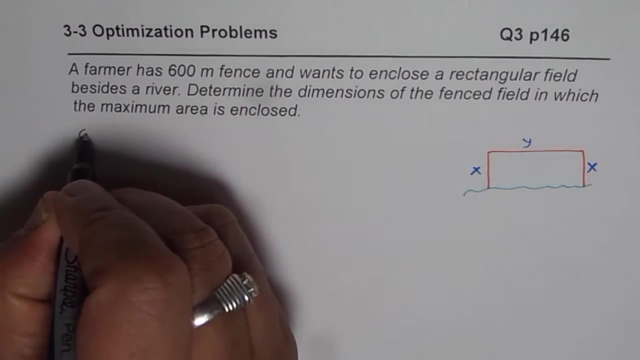 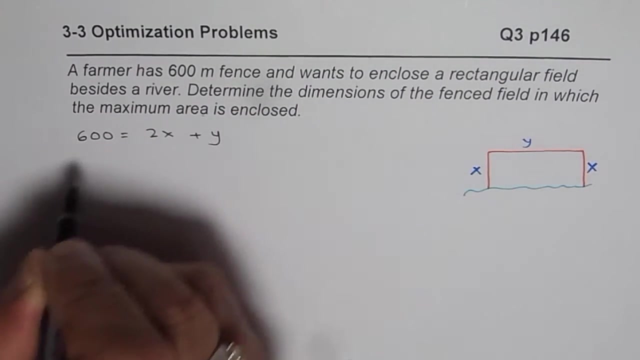 this is y and these two are x, right? So the width is x and the length is y for us, So that is how the diagram should be. And now what we know here is that there is a 600 meter of fence. that means 600 should be equals to x plus x, which is 2x plus y, or we can write: y is 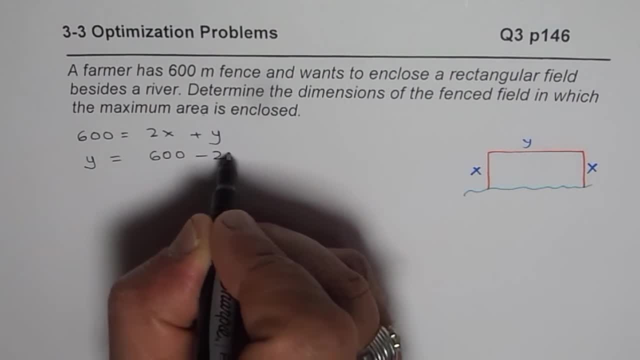 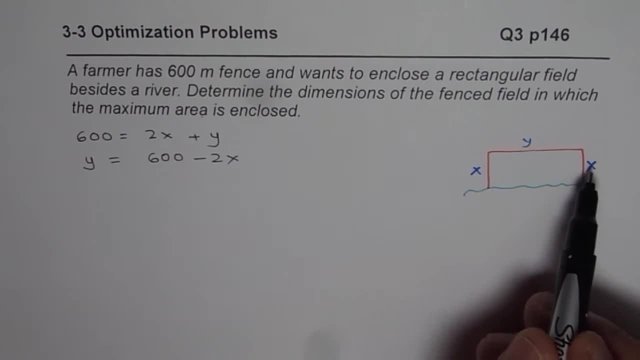 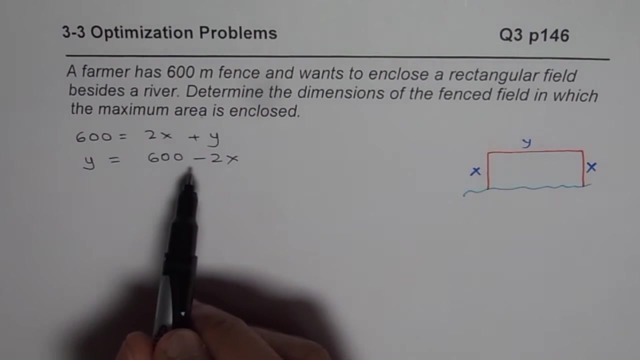 equals to 600 minus 2x. Now, with these statements, what we get is relation of one variable in terms of the other. So in most of the questions which we are going to work with, that should be a first step: Develop a relation between the variables, whichever you define, So in this case, width and 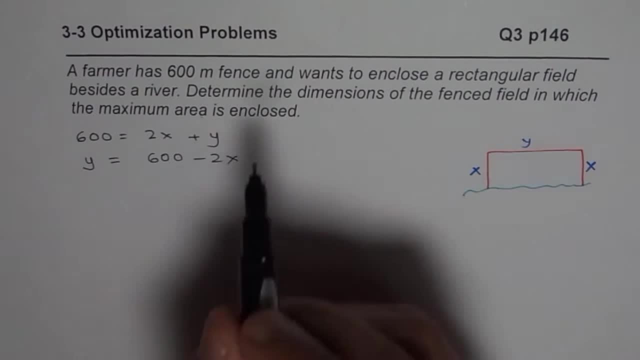 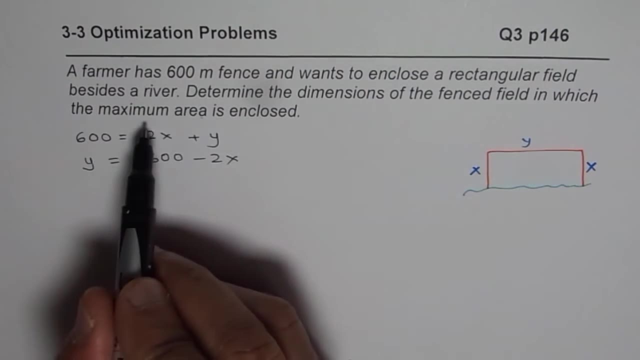 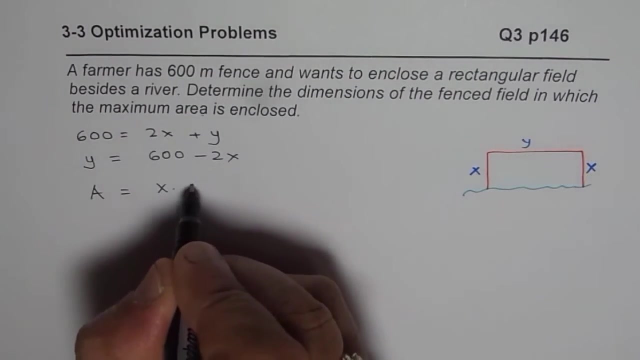 length are the two variables represented by x and y. Now what do we need to do? Determine the dimensions of the fenced field in which the maximum area has to be enclosed. Now, area of this field is what? x times y? right, x times y. We can now write y in terms of x, so we get area in terms. of x, So we can write x times y. Now we can write y in terms of y, So we get area in terms of x, So we get area in terms of x. Now we can now write y in terms of y, So we get area in terms of. 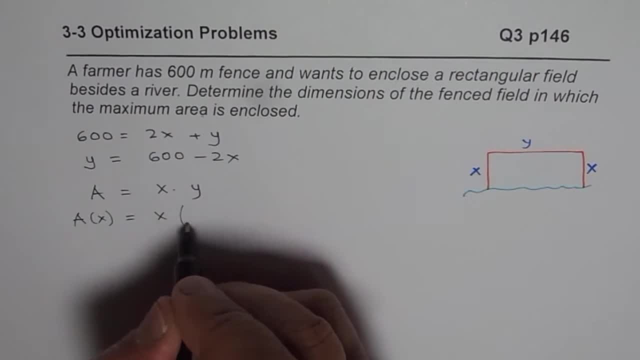 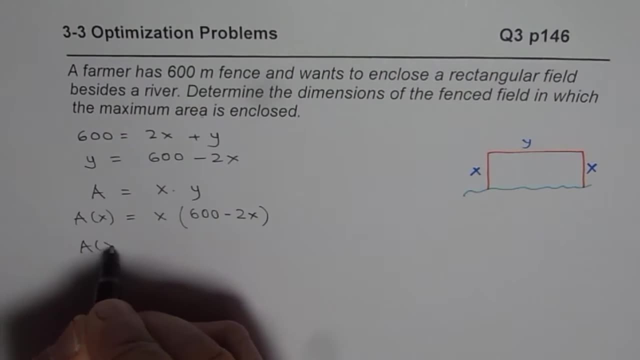 x as a function of x, So which is 600 minus 2x. At this stage it's a good idea to always expand this. So 600x minus 2x square becomes your equation for area. To maximize area we need to find the critical number, So find derivative of this expression, So derivative. 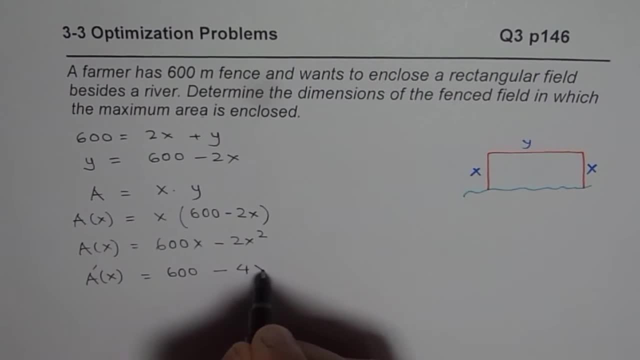 will be 600 minus 4x. Critical number is when the derivative is 0. So we will equate the derivative to 0.. So 0 equals to this. That means 600 minus 4x is equal to 0.. When will 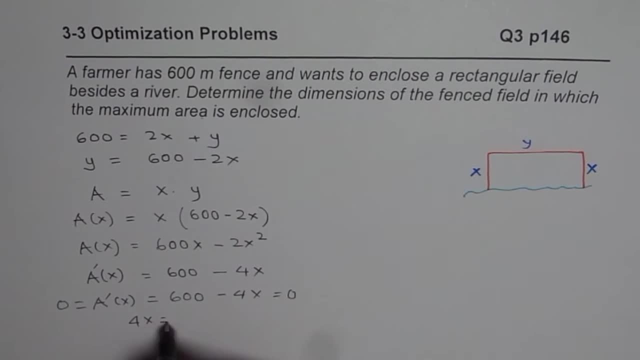 that be 0?? It will be 0 when 4x is equal to 600, or this implies, when x is equal to 600 by 4.. So half is 300, and then half of that is 150.. So what you get here is that the critical. 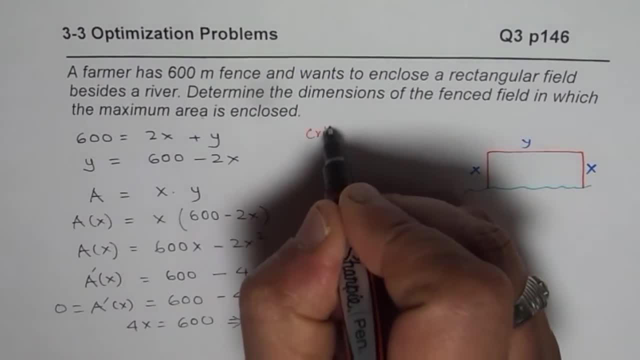 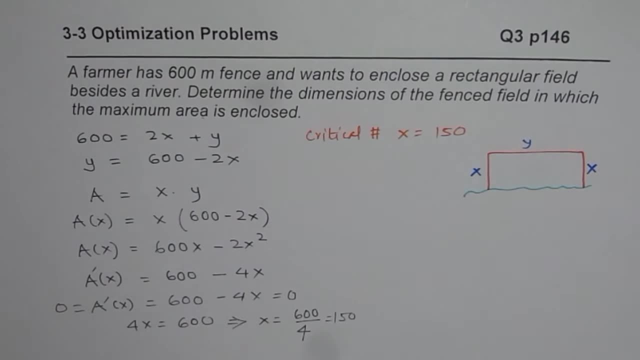 number for you is. let's write down the critical number. Number is x equals to 150.. Now, as you can see in this particular case, what could x be? So x could change from 0.. x could change from 0.. To what? So this cannot be negative. Do you see that? So the value of x could be if you? 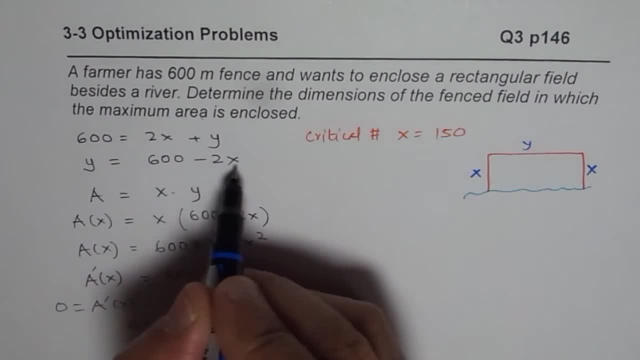 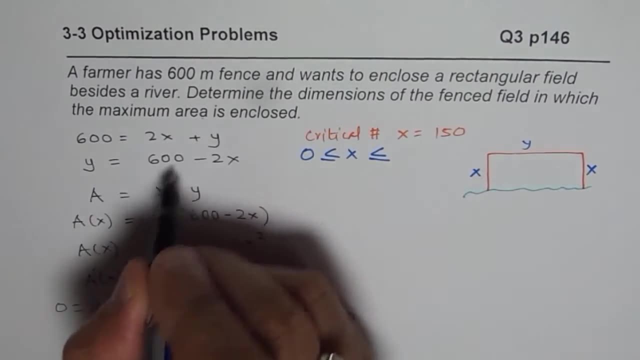 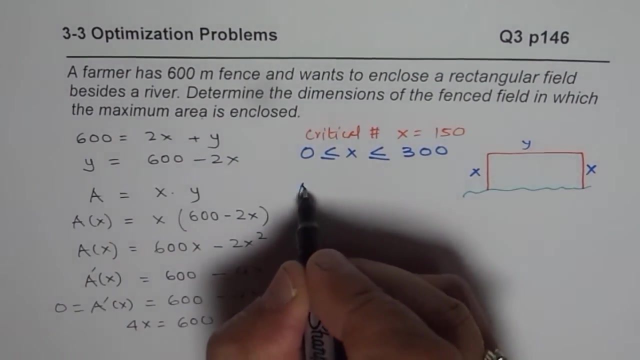 can see, from this particular expression we get the domain for x. So x could be greater than 0 or could be less than 600 divided by 2, which is 300.. Is that okay? If I substitute these values, I will get my area So to find whether this is maximum or not. we will find. 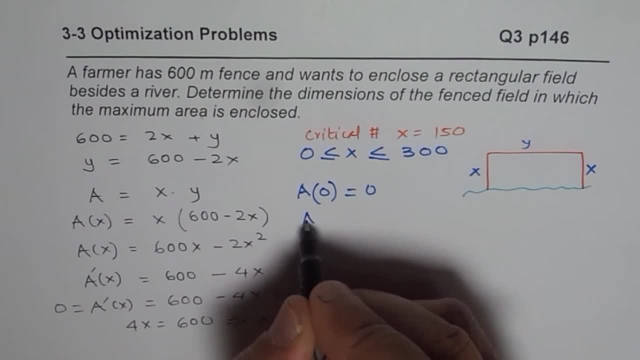 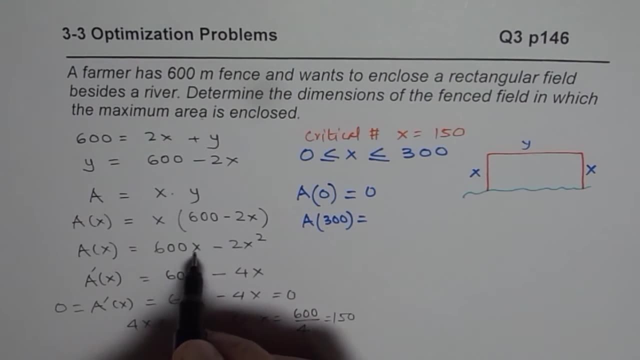 area for 0.. So x is 0. So which is 0.. Area for x equals to 300, which will be equals to 600x minus 2.. So if I write 300 here, this expression will be 0, right, So that will also give me.